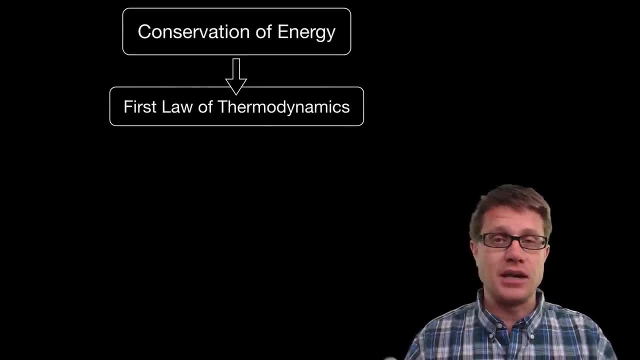 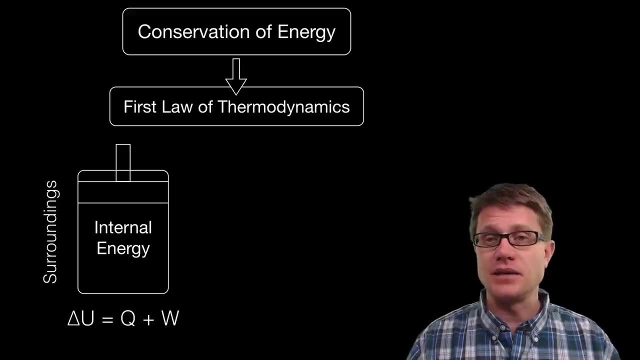 And so a part of the conservation of energy is the first law of thermodynamics. Energy can neither be created nor destroyed, But we are going to study how this applies in a typical idealized gas in a piston like this, And so our equation is delta U, so that is. 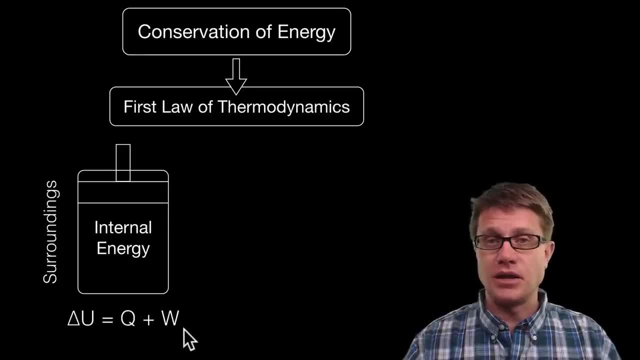 the change in internal energy is equal to Q plus W. Q is going to be heat and W is going to be water, And so we are going to use this equation to calculate the temperature of the piston to work, And so we can add energy to this system, this internal energy, by heating. 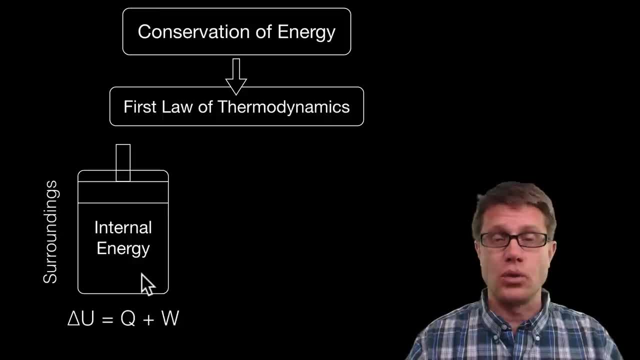 it up, Or we can apply a force over a given distance to it. We can do work on it, And so what we are looking at is how energy can be transferred from the surroundings into the system and back again. Now we are not going to lose any energy. Remember the energy. 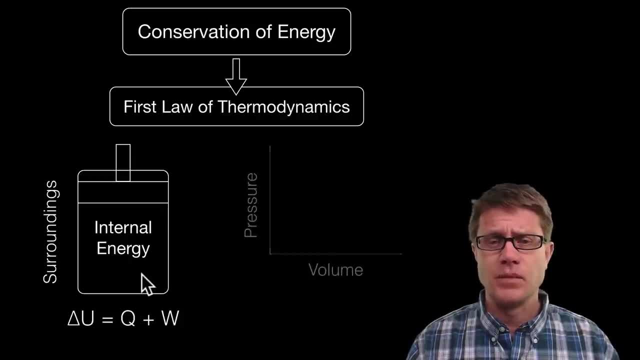 is going to be conserved, And a good way to measure this using a piston is to graph the pressure and the volume over time. And so we are going to start with the piston kind of relaxed And we are going to have a really high volume And we are going to have a really 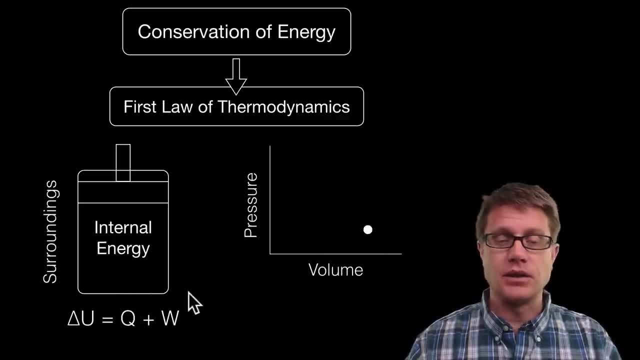 large volume here, But it is going to be a relatively low pressure And then I am going to compress that piston. So the surroundings are going to do work on the system And as they do that, you can see we have an increase in the pressure inside. Now we did it slow. 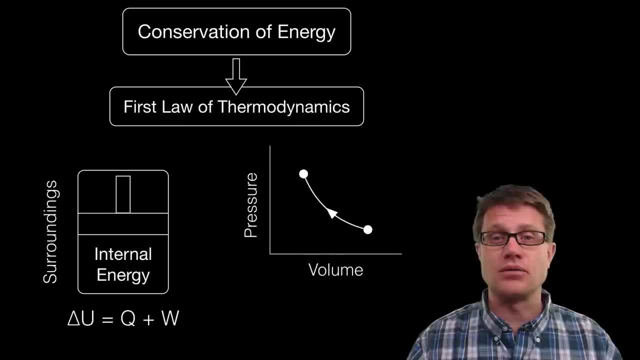 enough that we are allowing that temperature to stay constant throughout that whole process, And so what is neat about a pressure volume diagram is the area under that curve is going to be the amount of work that we do Now. a common mistake in physics is to figure out. 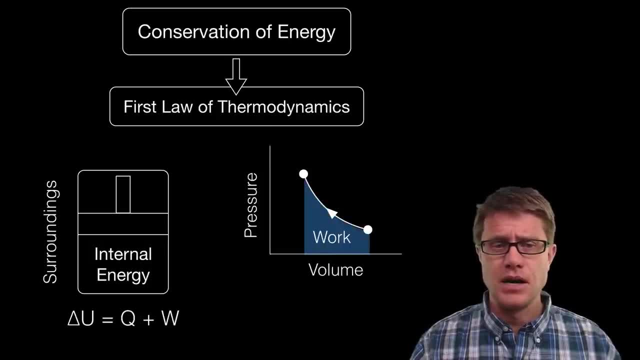 who is doing the work? Is it the system or is it the surroundings? And so in any piston like this, the area under the curve is the work being done by the gas, And so you can see that we are going from right to left, And so this is negative work. And so what? 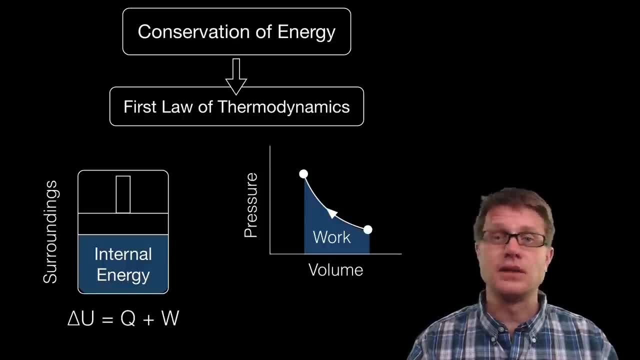 is work being done by the gas, It is negative work. Well, if it is negative work of the gas, that means it is positive work of the surroundings. We are adding work on the system, And so we are increasing the amount of internal energy on the inside. 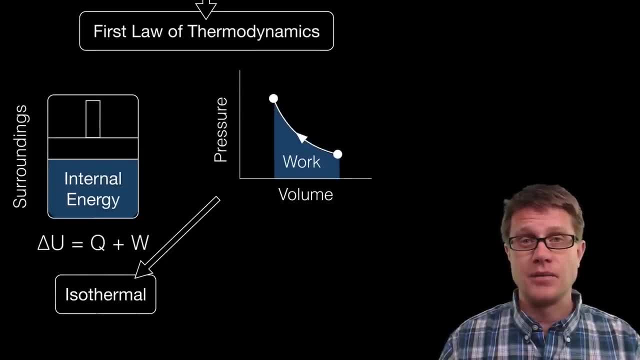 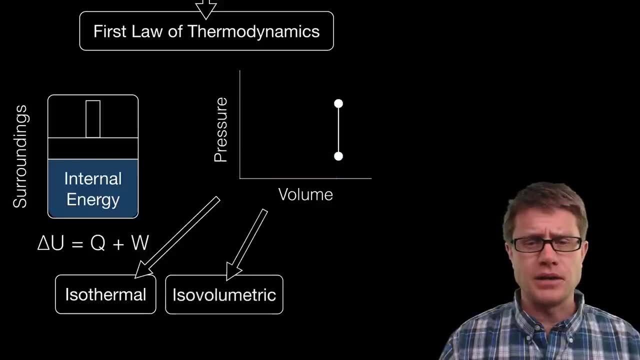 This would be an isothermal process, since we are keeping this temperature the same. Now, in physics one and two, you do not have to do calculations, You just have to know qualitatively what is going on. But we could have a different process that we will model here. It could be isovolumetric. 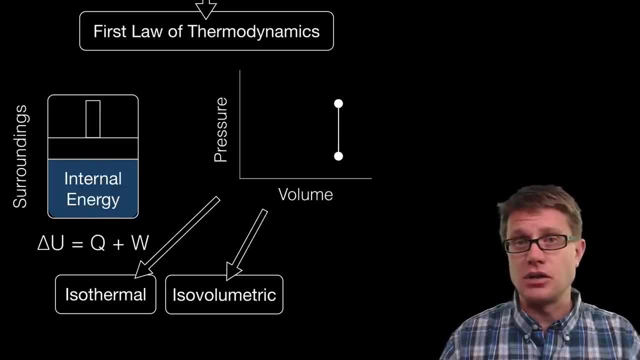 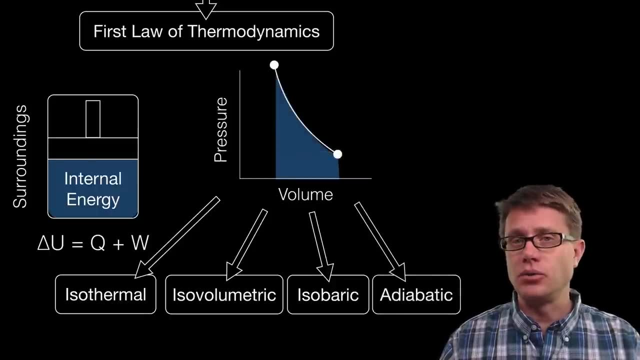 We could lock the volume of that piston And we could just add energy. through heat We could have isobaric when we keep the pressure the same, Or in the fire piston we can do adiabatic cooling or heating. So that is when we are doing it so quickly that we are not. 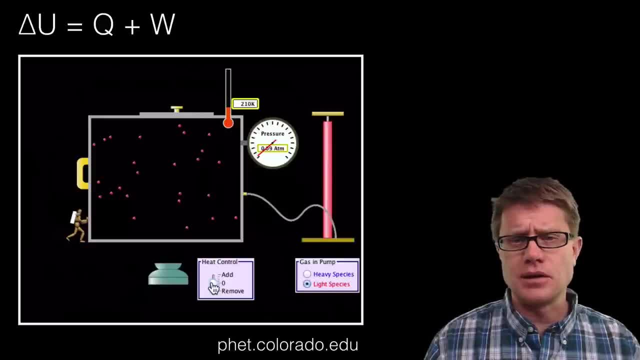 allowing heat to kind of move in and out. And so let's start with a little simulation here. This is a PHET simulation. We have got the gas molecules on the inside, We can add heat right here And then we can push back and forth on the piston on this. 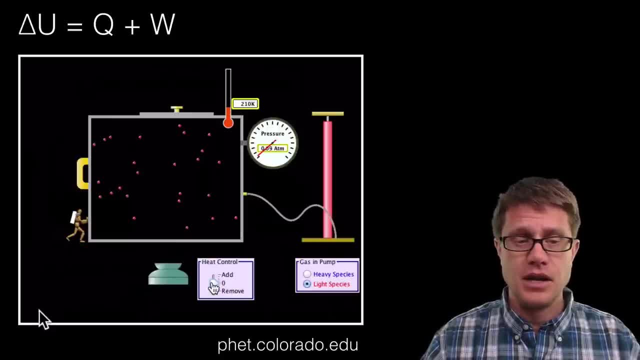 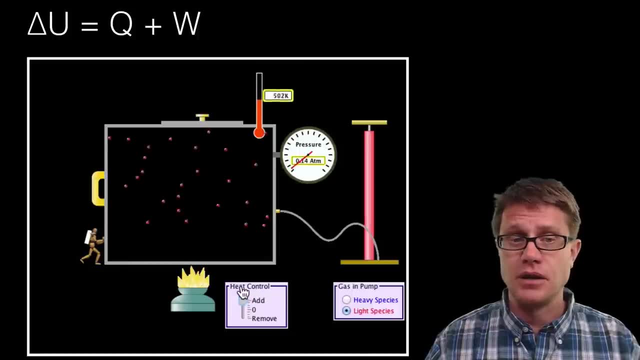 side. so we can do work. We can apply a force for a given distance, And so let's watch what happens when we run this simulation. The energy is in the molecules on the inside. What happens is I add temperature to it, I am increasing their speed, and so I am increasing their energy. 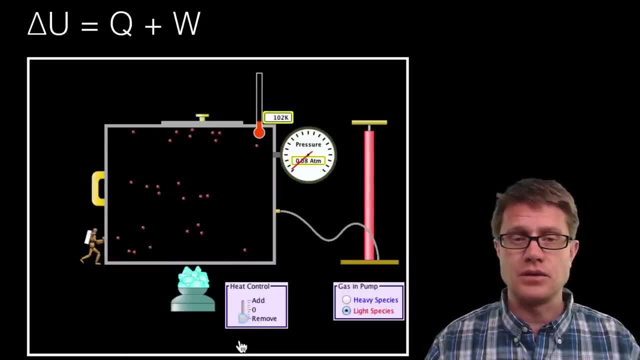 Energy of the system increases. If I cool it down, energy of the system decreases. How else could I add energy? Remember it is W, It is work, So we could push in on it. What is happening to the pressure and therefore the energy on the inside? It is increasing And now that total internal 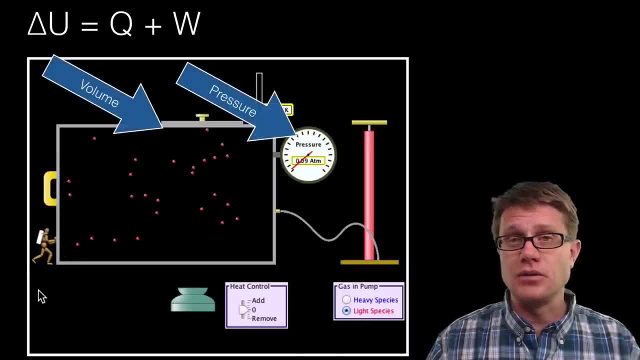 energy is decreasing over time, And so it is nice to be able to use a simulation, But the two things that we can measure are the volume and the pressure, And so if we just keep track of the volume and the pressure over time, we can figure out what kind of a 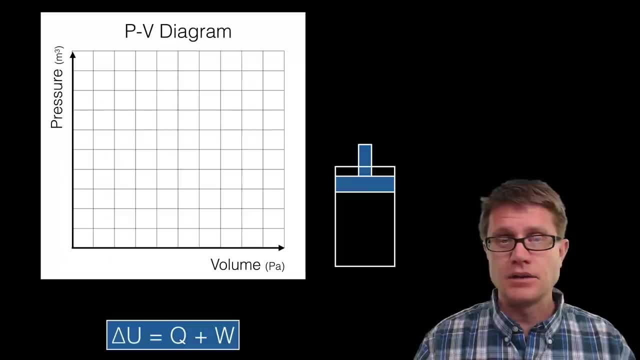 process is going on, And so this is a PV diagram. And so let's start with an isobaric process. In an isobaric process, we are going to keep the pressure the same, But we are going to be able to change the volume over time, And so a way. 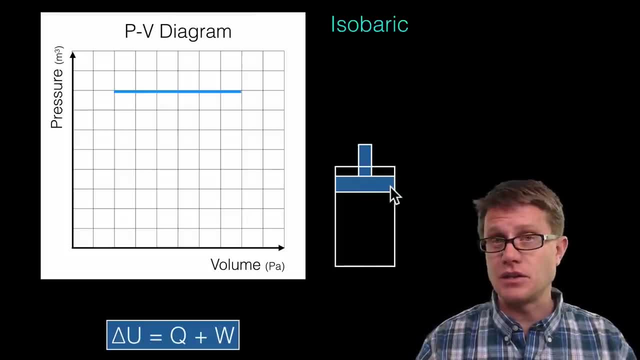 to do that is allow this piston to move in and out, And so we can change the temperature. What is going to stay the same? It is going to be the same pressure on the inside. So that piston is going to move back and forth, But we can add energy into the system or we 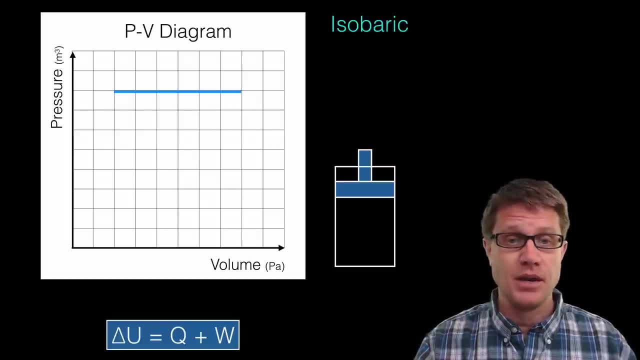 can pull energy out. Since it is free to move, the pressure is going to stay the same, And so if you see on a PV diagram this horizontal line, then you know it is isobaric. What else could we do? We could do iso-volume measurement. What else could we do? We could do iso-volume. 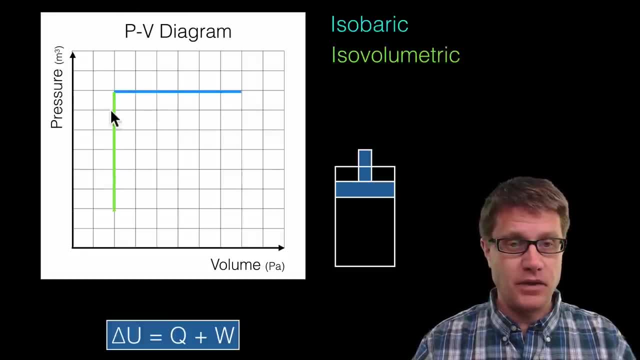 metric. What does that mean? We are going to keep the volume the same. You can see, the volume is always the same, So it is just going to move back and forth on here. We are going to increase or decrease the pressure, And so what would that look like using our piston? 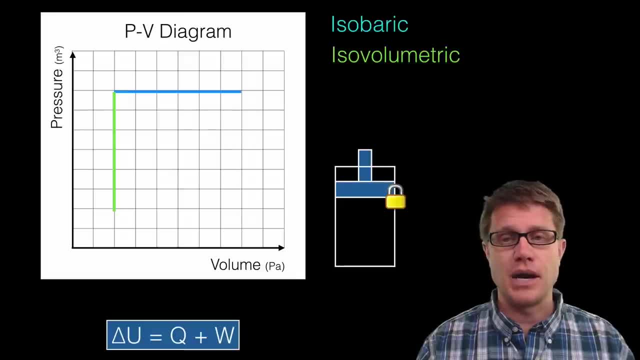 We are going to lock it in place. Now we can add temperature. We could pull that temperature out. We could also have isothermal. Iso-thermal is always going to look a curve like this. This would be an isothermal curve. And so how do we do that? with a piston? Well, we will. 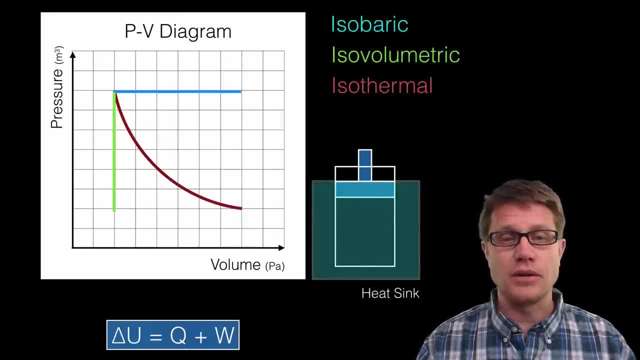 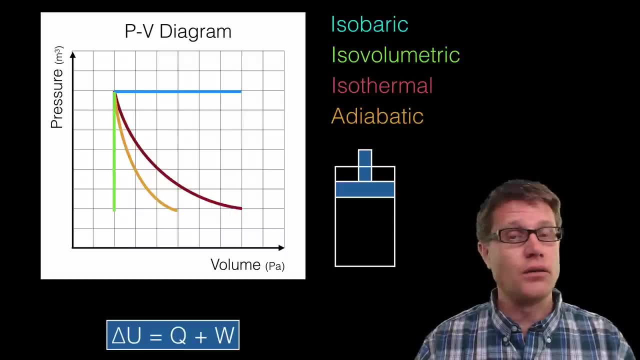 use something like a heat sink where we can keep the same temperature throughout that whole process, And then, finally, we could do adiabatic. That is where we either pull it out or move it in really, really quickly. It is so fast that we cannot lose temperature to the surroundings. 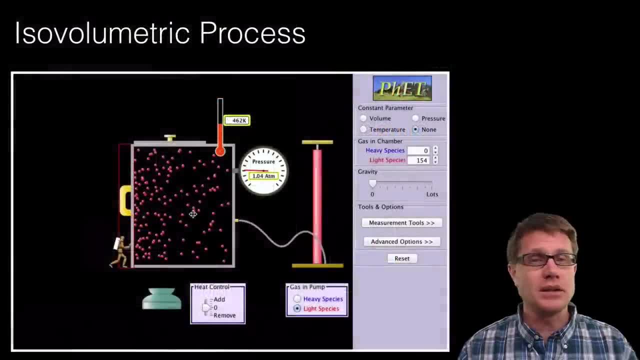 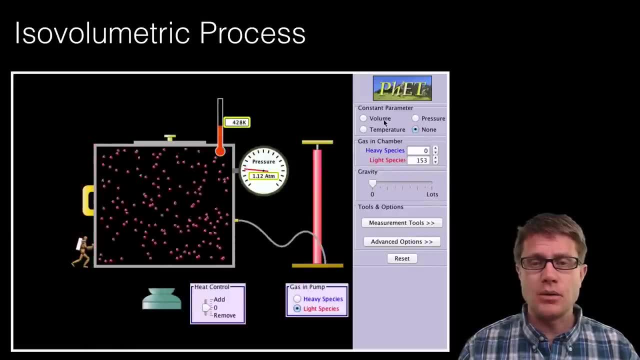 and you are going to get a curve that looks something like that. Okay, So let us kind of model those using this PHET simulation, And so let me kind of get this thing going. There we go, And so now what we are going to do is we are going to keep the volume constant. 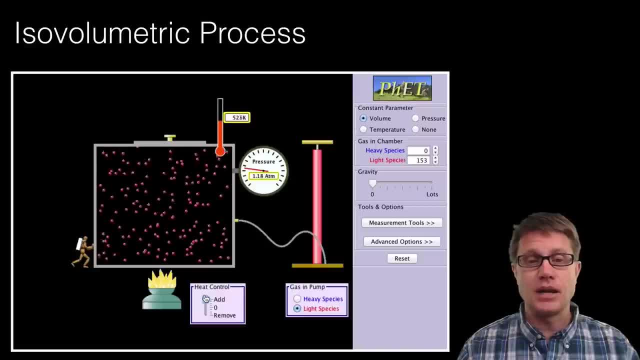 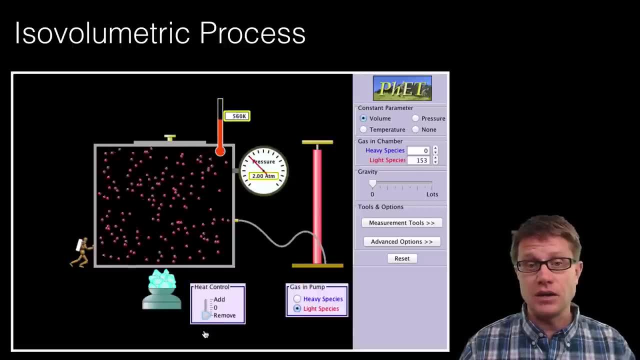 So we have locked it in place. How do we get energy into the system? We could add heat. As we add heat, we increase temperature Pressure is going to go up. Let us say we add ice on the bottom, We are going to pull energy out of it. Heat is going to flow from the system. 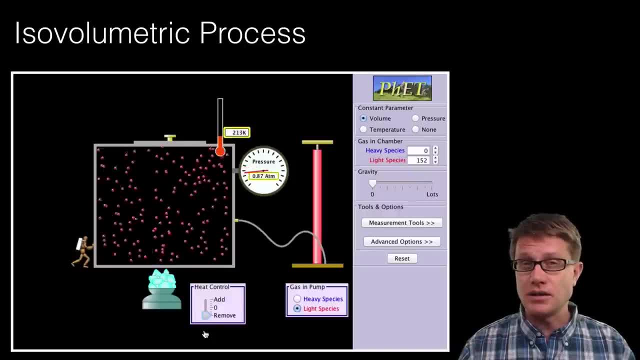 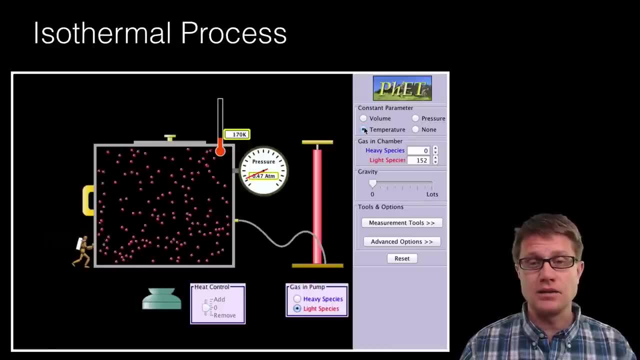 to the surroundings And the pressure is going to decrease. What is staying the same that whole time? The volume is going to stay the same. For the second one, let us keep the temperature constant now. So we have got a constant temperature. So you can see that I cannot even change my 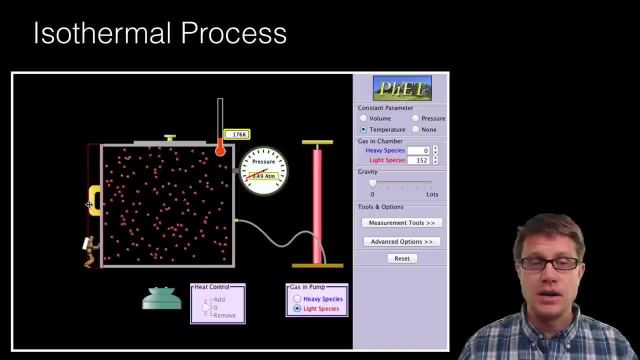 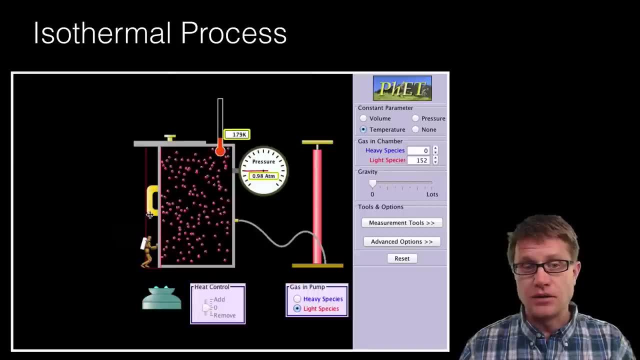 heat controls here. So how am I going to get energy into or out of the system? It has to be through work. So if I apply a force from the outside, what is happening to the pressure on the inside? It is going up. If I do negative work from the outside, what is going to happen? 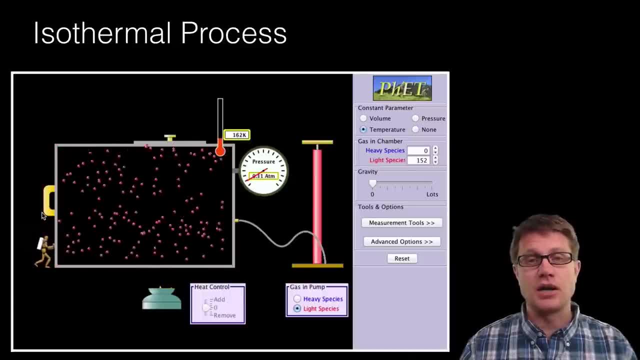 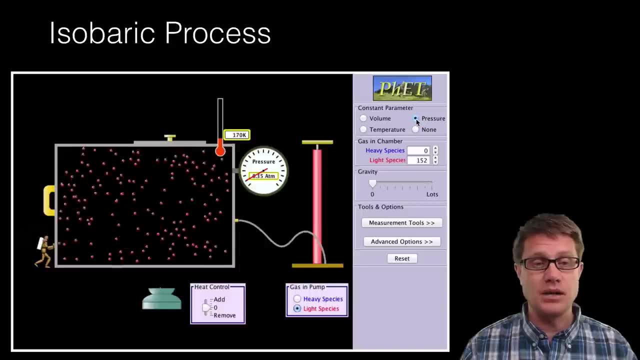 to the pressure, Pressure is going to drop off, And so we are going to get that nice curve on a PV diagram. And then, finally, we can look at an isobaric process. In an isobaric, we are going to keep that pressure the same. What does that mean? This piston can simply 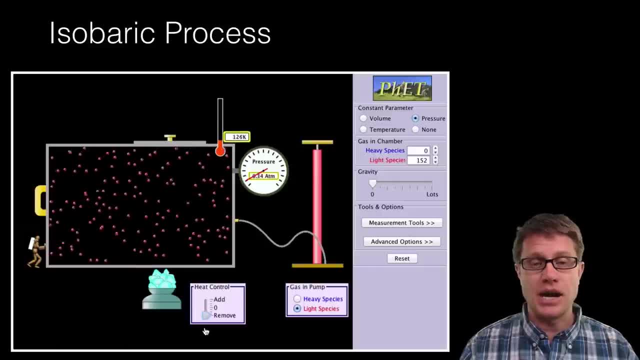 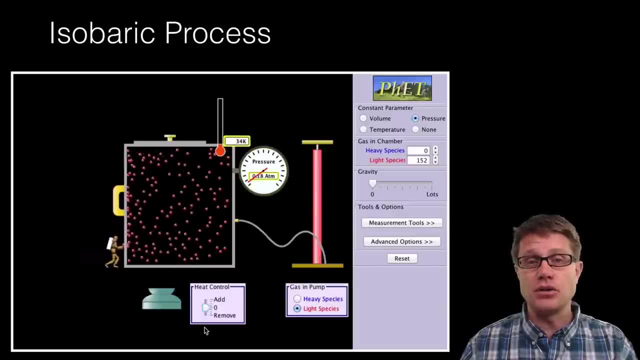 move back and forth. It is going to be the same pressure exerted by the gas. If we cool it down, those molecules move slower. The piston is simply going to move in If we were to add temperature to it. as we increase temperature, that we are adding temperature or heat into. 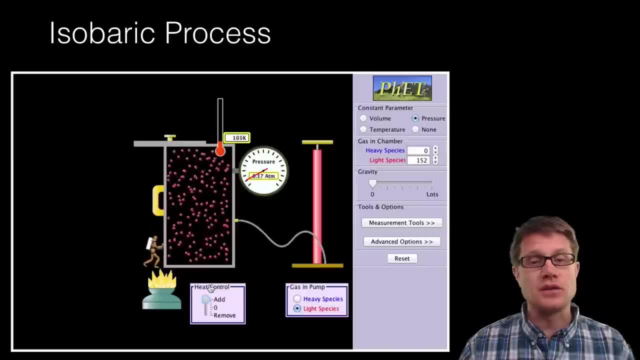 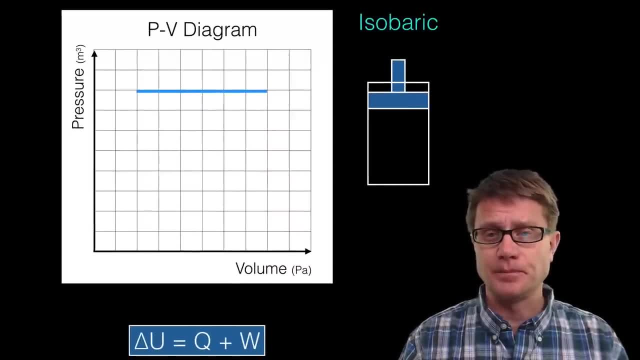 the system. what is going to happen? Those molecules are going to move quickly, They move slowly, But since the pressure remains the same, the piston is going to move out. And so what would the PV diagram look like in an isobaric process, Since that piston, 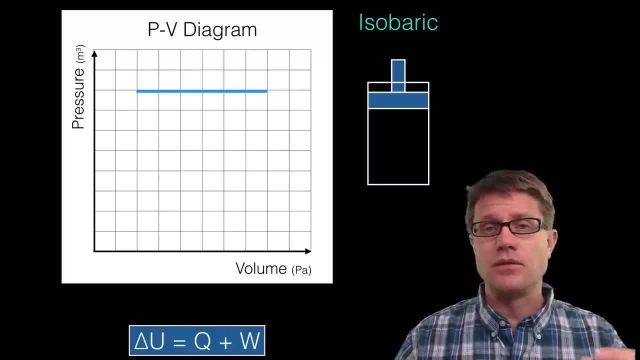 can move back and forth, the pressure is always going to remain the same, And so the volume is going to change over time. And so, remember, the area under a pressure volume diagram is going to be the amount of work that we do, And so, since we are taking a large volume,